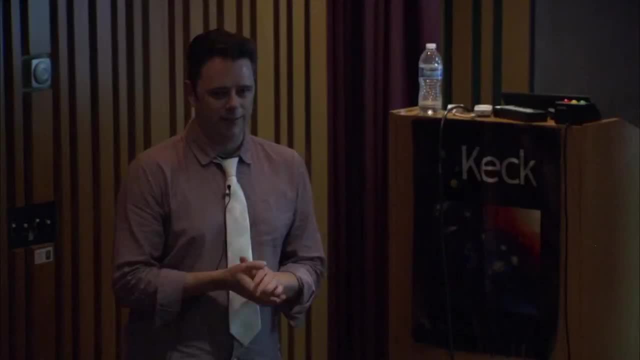 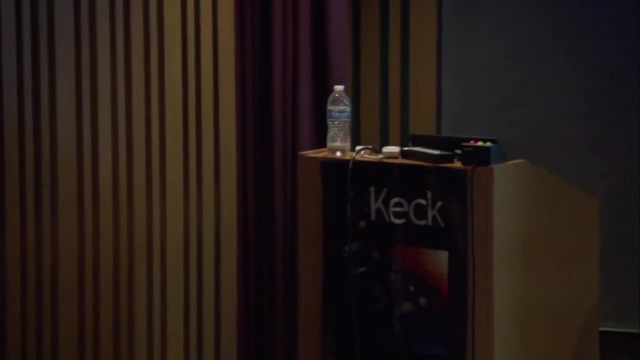 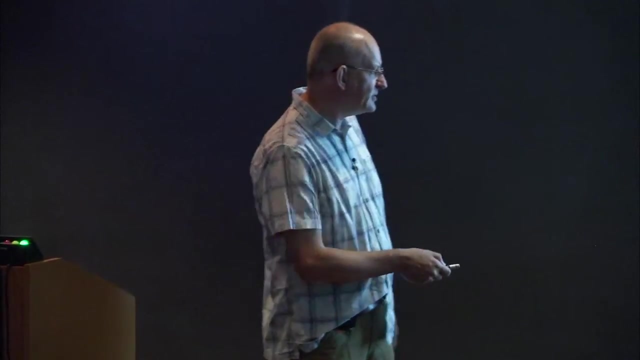 So our morning talk is really focused on the ocean side. Our mid-morning talks will focus more from the glaciological perspective. Thanks, very much, Thank you. So I'd like to acknowledge my co-workers Steph Cornford, Rupert Gladstone and Dan Martin, who works at Lawrence Livermore. 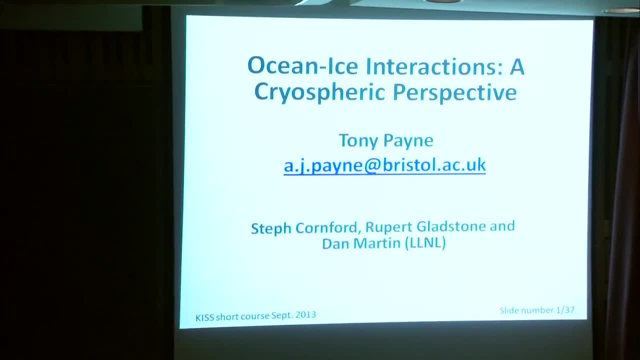 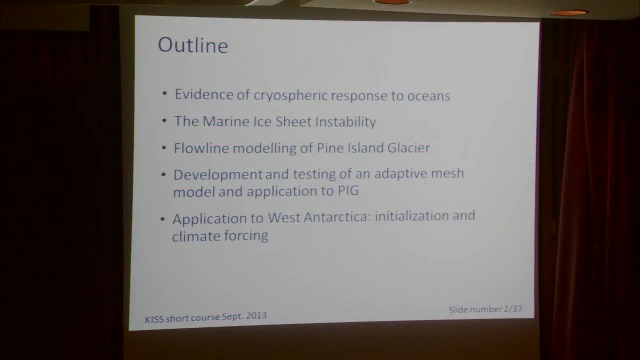 And many of the results that I show are due to their work. Outline of what I'll talk about, some evidence of why we believe the oceans are important in generating the changes that we observe in Antarctica. The elephant in the room is the marine ice sheet and stability. 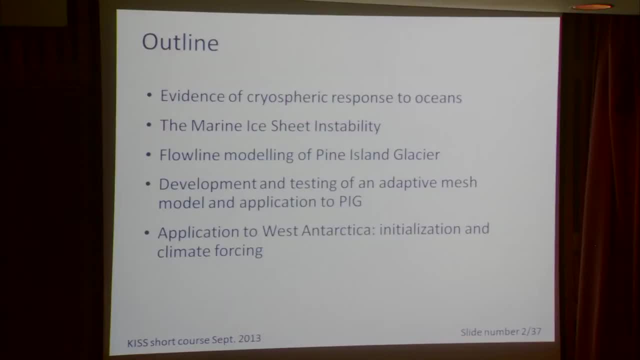 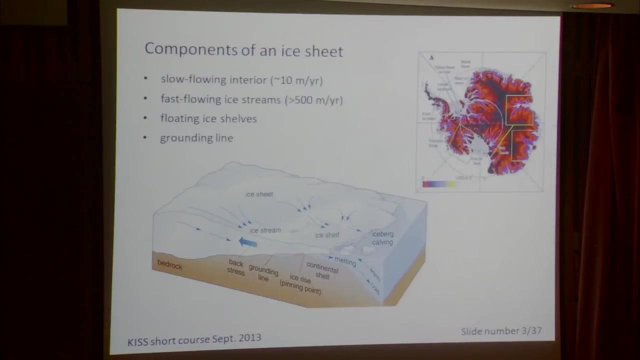 I'll talk about that briefly And then I'll talk about specific modeling of Pine Island glacier, More recent work on ice sheets, How one ought to model the grounding line, in particular using an adaptive mesh system, And then the extension of that work to the whole of West Antarctica. You've seen a figure. 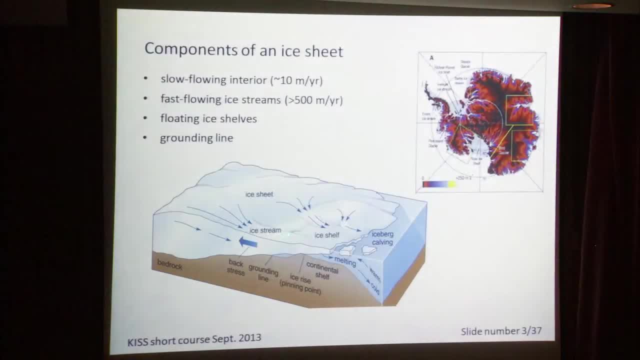 like this already Key vocabulary- ice stream and grounding line- is primarily what I'm going to be talking about today. You know what ice shelves are. Ice streams are zones of fast flowing ice within the ice sheet, And here's an illustration showing in the lighter in. 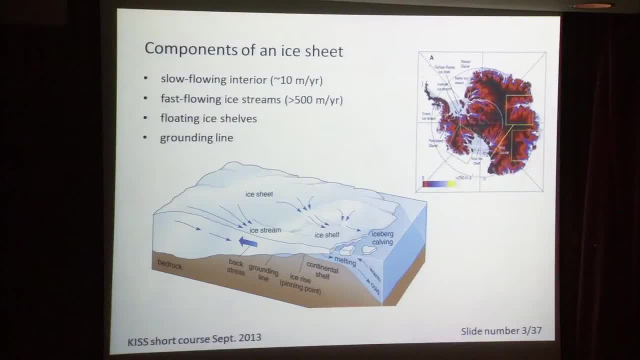 red and blues, fast flow, And that could be of the order of kilometer per year, for instance. And these ice streams are embedded in the ice sheet, where typical horizontal flows are of the order of, say, 10 meters per year And much of what I talk about much. 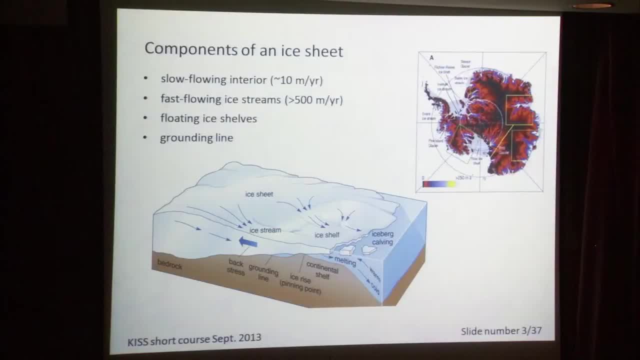 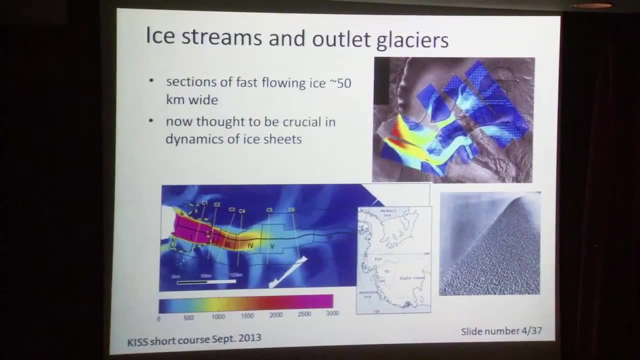 of the observations are related to ice streams, rather than this passive, fairly slow flowing ice sheet. Here's some imagery of ice streams 40 to 50 kilometers wide. Here's an aerial shot of one. They're characterized by very abrupt shear margins. So there's at least an order of magnitude difference in the horizontal. 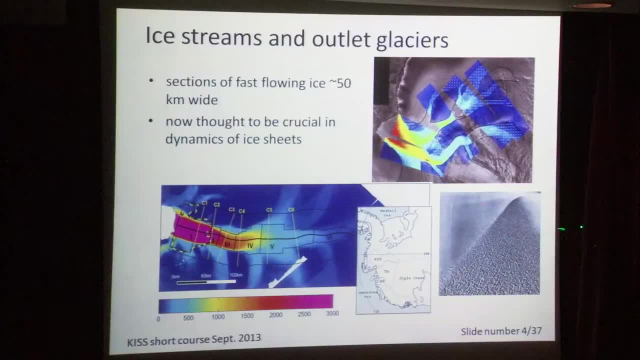 flow here slow flow, very smooth ice surface, crevassed ice surface: here fast flow. And this is the type of imagery that I'm sure Eric will show later on of showing the velocity as measured by from space using a technique called interferometry. 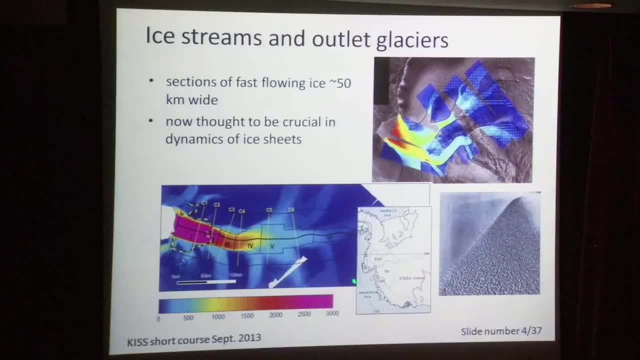 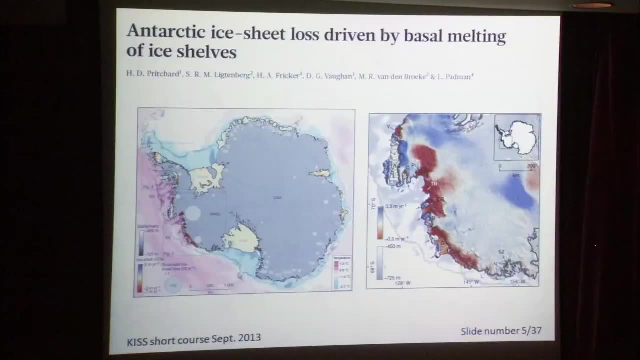 For a particular ice stream in Antarctica. This is Pine Island, which is our poster child, and we'll return to Pine Island quite a bit. Now you're all here because you believe that the oceans and the ice interact, So I'm not going to go through a huge amount of evidence as to why we believe that is the case. This 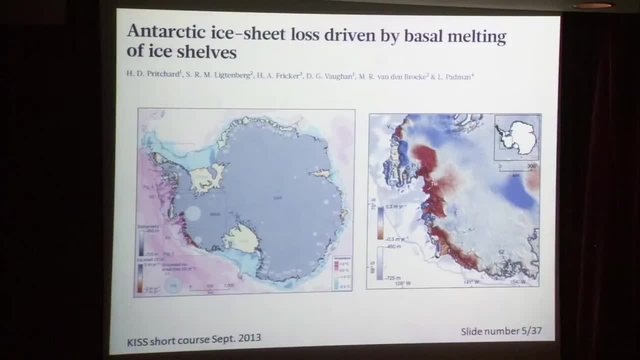 is just an image from Amos Pritchard's Nature paper of a couple of years ago, where he shows in red ice shelves that are thinning, based on altimetry. This is a LIDAR system, space-borne LIDAR system: Red ice streams that are thinning, Yellow ice shelves, rather, that aren't doing. 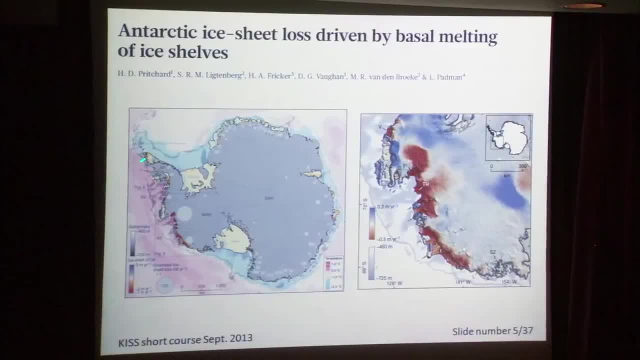 very much And he's very suggestively overlaying observed ocean temperatures And we of course notice that the coincidence of warm ocean waters with thinning ice shelves. In this panel we take the signal, the signal. 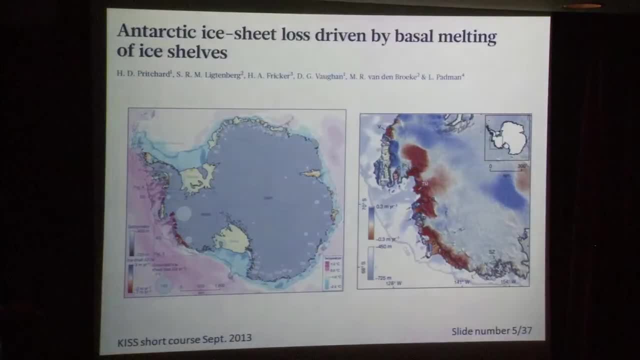 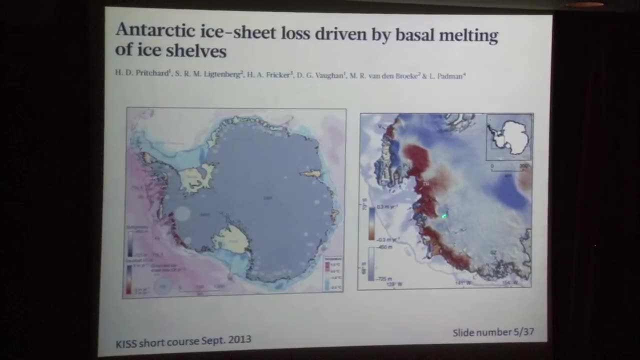 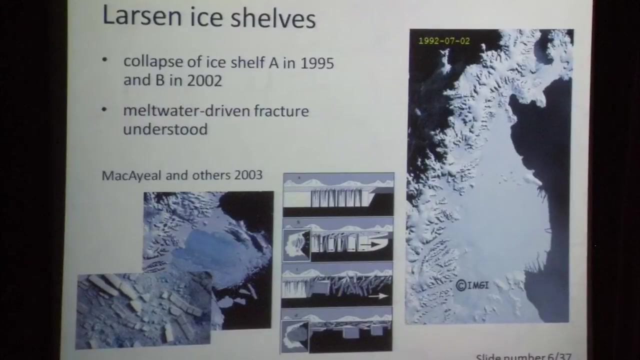 from the ice shelves here and look how well it corresponds to thinning in the grounded ice. Pine Island- its neighbor Thwaites Smith's Glacier down here- gets here. Before I go on to talk about Pine Island, I think it's worth talking about the Larson. 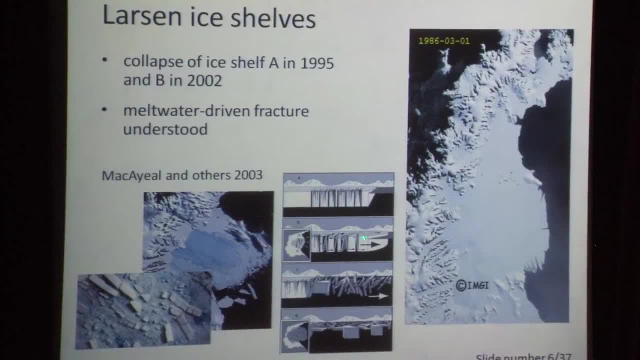 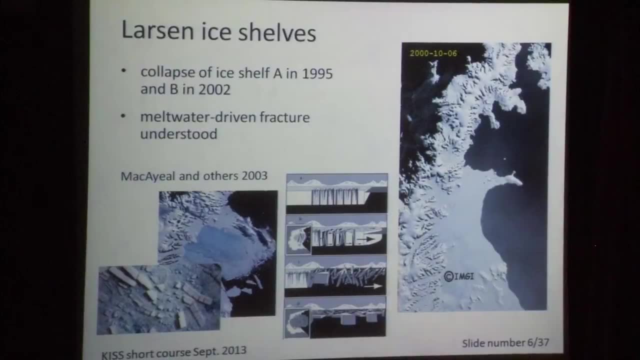 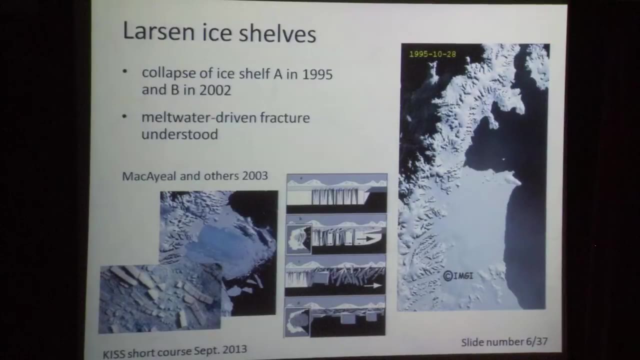 ice shelves and their collapse. These are ice shelves: the Antarctic peninsula, Here's the peninsula, South America- Okay, up there. and they're collapsed in 1995 for A and 2002 for B. Now, although the mechanism may be something to do with ocean warning, it's primarily an atmospheric signal, and I'm going 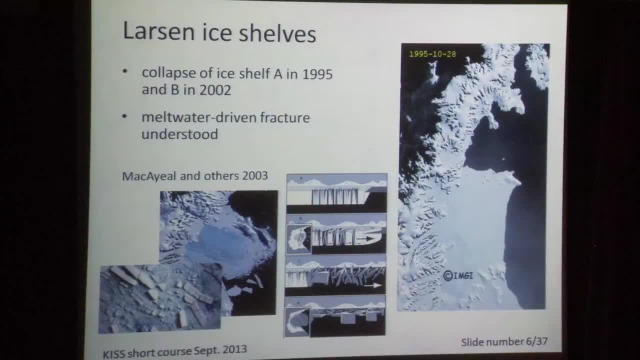 to use Larson in particular, as a natural experiment. So we know that on a particular period of time, the ice shelf disappeared- and you'll see a couple of papers in a moment that use this event as a laboratory, as a test- and there's been a debate, a largely theoretical debate. 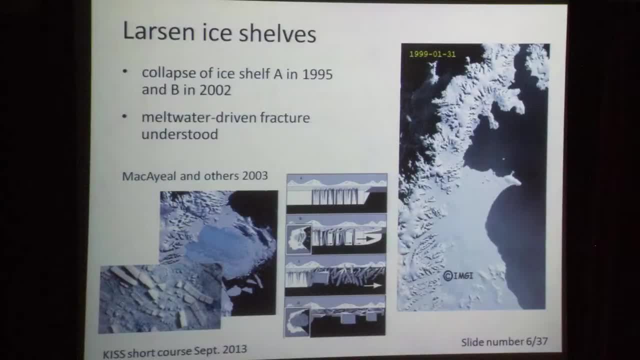 in glaciology that's lasted perhaps 30 years or more, on the degree to which ice shelves talk to the grounded ice that feeds them. So the question is: what happens if you get rid of an ice shelf and here an ice shelf has disappeared? so we can answer that question using observational data rather than 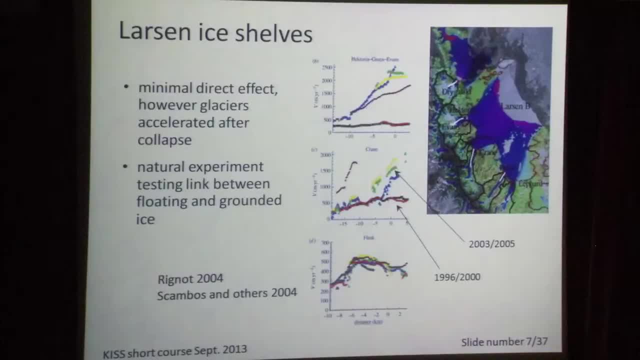 theoretical ice, And there's a couple of papers in particular that did this. so here we have the ice shelf again. these colors refer to velocity. here we have the mountainous spine of the peninsula and we're going to look at velocities in a number of glaciers that fed into the former ice shelf. 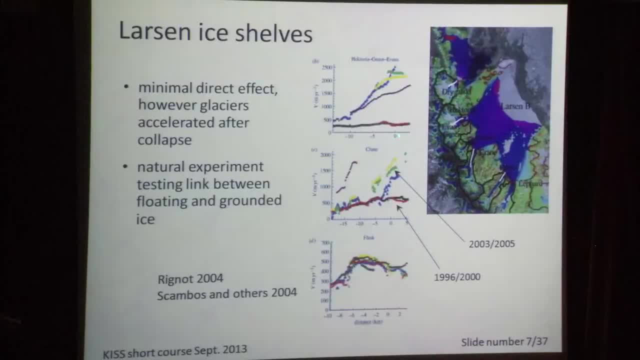 and these are the data: distance from the grounding line. so with the grounding line here, this is the ice shelf- we're going up glacier in this direction for all three of these glaciers and we have velocity here and the different lines refer to different years. so we have 96- 2000 in red and blue and then 2003, after the collapse, in reds, in yellows and greens. so you 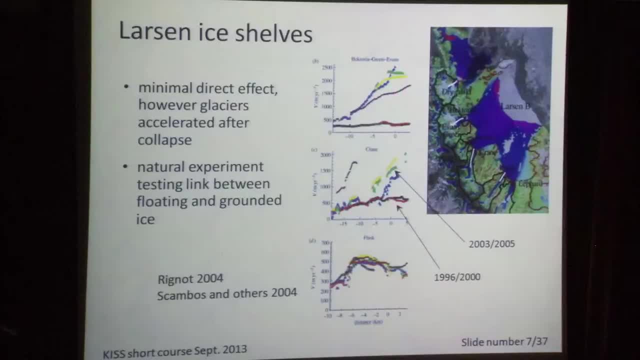 can see that for Hectoria Green Evans there's a very abrupt jump in velocity, and for Crane also. Now that's fairly convincing, but of course it could be that whatever caused the loss of the ice shelf caused the increase in velocity, so there was something else that caused both things to happen, and fortuitously. 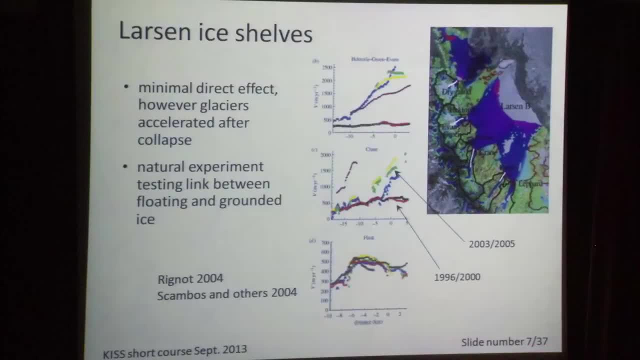 there's a natural control experiment as part of this, so it's a fantastic experimental design, and this portion of the ice shelf didn't collapse completely and flask glacier that drains into it didn't respond. so from this work we can say pretty convincingly that if you lose an ice shelf, you do affect the flow and the mass loss. 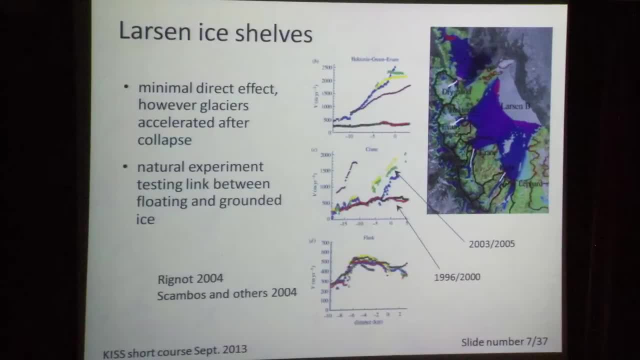 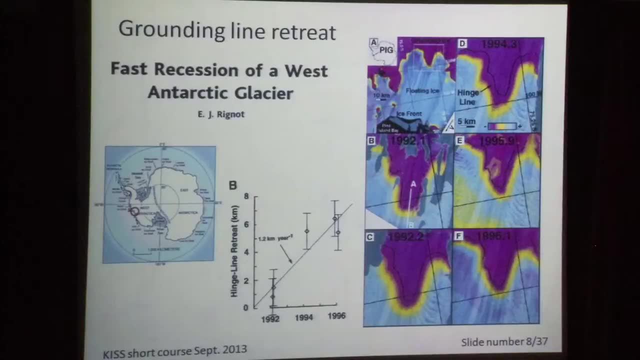 from grounded ice which, as i say, was a subject of a very long and sometimes acrimonious debate within glaciology up until this point. So we've dealt with blast and b and we've taken from that. but yes, you can lose an ice shelf and that will affect the grounded ice and the amount of mass that's lost from the ice shell. 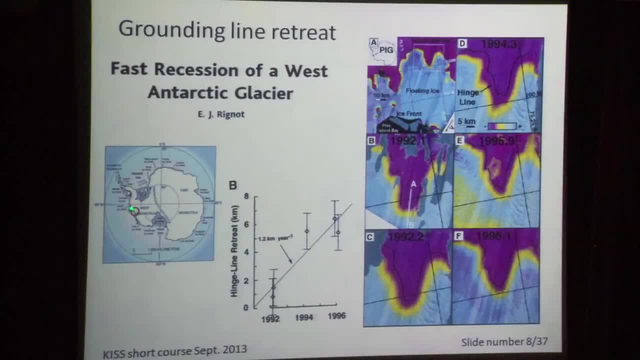 so this is our test, if you like. like Now we're going to try that to the far bigger system. Last, and although it's significant, the loss of the ice shelf and the increase in discharge wouldn't affect sea level hugely. What's more important is Pine Island and the Thwaites Glaciers over here. Eric will probably. 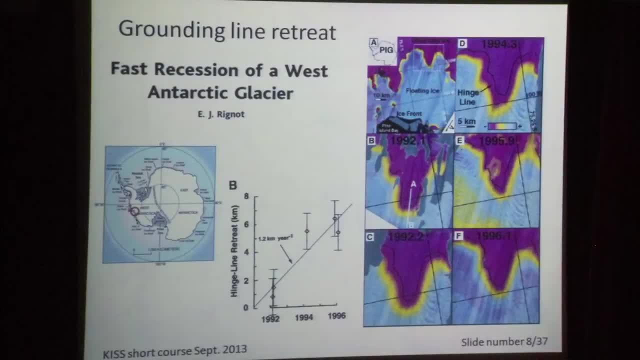 talk about his earlier work. that was the first to identify that things were happening in Pine Island by mapping the grounding line, the line that separates ice resting on bedrock from floating ice shelf ice. There's a series of images here that map the progressive retreat. 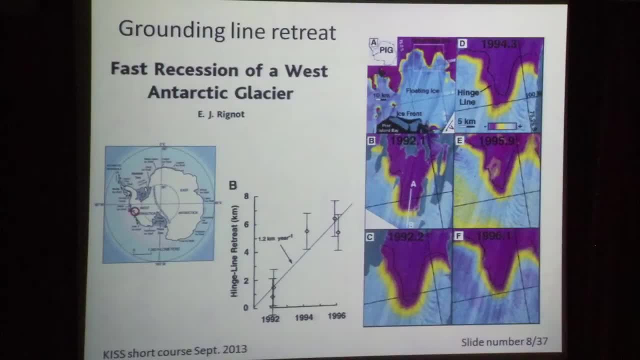 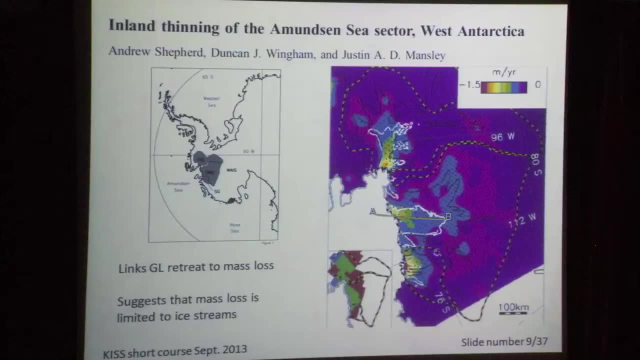 of this grounding line. That was the first indication that things were up. Shortly afterwards, another satellite-based technique, altimetry, was used to map the change in surface elevation of the ice streams in this sector. We can see that here's Pine Island. We know the grounding. 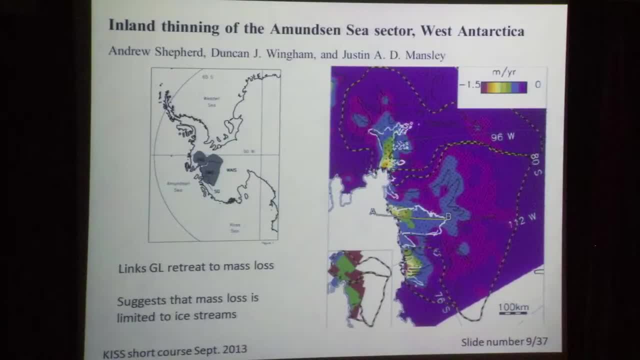 line is retreating. Coincidentally, mass is being lost and the surface elevation of the ice stream is deflating. That's also true of parts of Thwaites and the Smith Glacier. here There's two lines of evidence there that are starting to tie up very nicely. The third line of evidence. 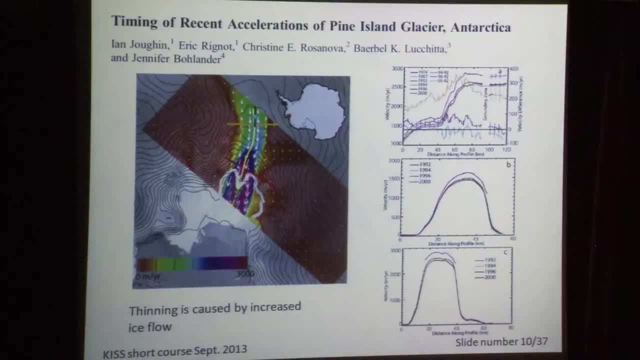 was provided by Ian Yockin who, again using satellite interferometry, maps the velocity of Pine Island, Glacier. We can see only that the temperature has increased. Well, there was some actual photographic engineering done which shows that the temperature did increase. We can see that the temperature. 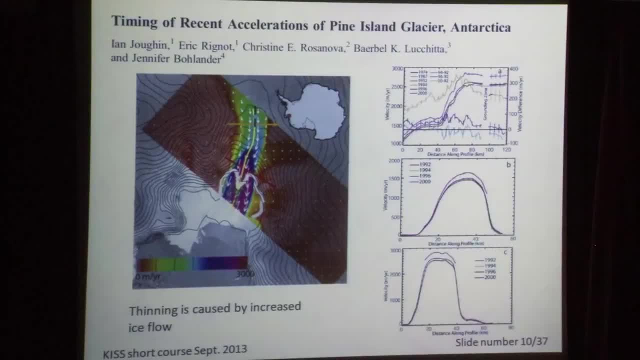 has increased during this period. We have grounding line retreating, mass being lost and mass being lost because the glacier has accelerated. All those are pretty well-agreed. Now we know that in this particular area of Antarctica, air temperatures are sufficiently cold. 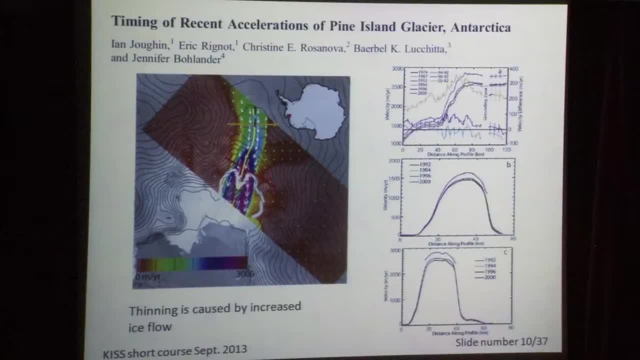 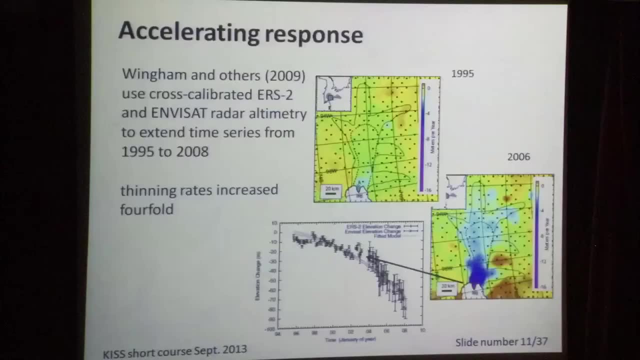 not the case for Larsen, where you had large amounts of surface melt. it's something else and the obvious candidate was: the oceans or is the oceans? are the oceans? More recent work by again using satellite altimetry by the UCL group in. 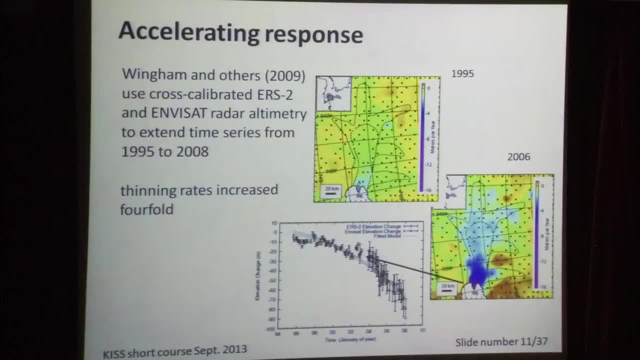 in London showed that not only is this trend continuing, it's increasing. So here we have the original data set that caused concern. and again, colors refer to thinning rates. So the bluish colors are roughly, let's say, two meters per year. thinning green yellows: not much happening. That was in 95, using this. 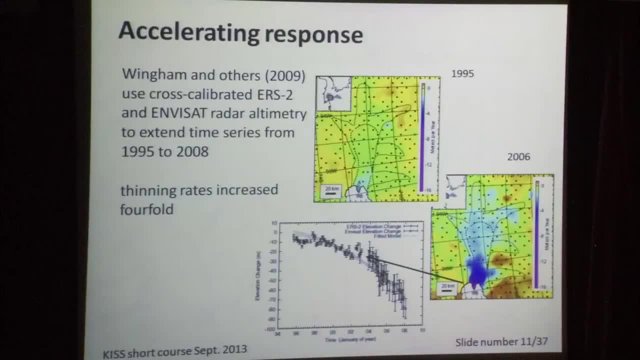 slightly different satellite but similar technique In 2006. you can see that that thinning has accelerated to the point where we're now down over a 10 meters per year thinning, And here's a time series going from 94 through to 2010 of the elevation change. 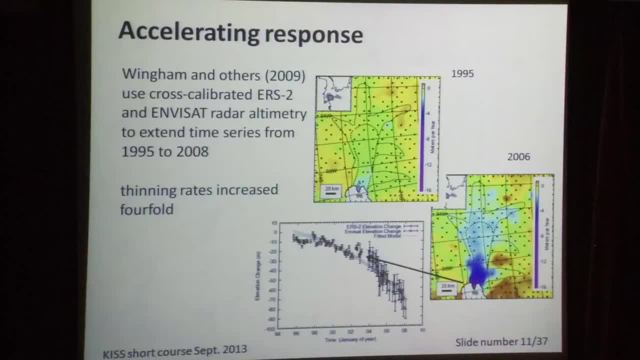 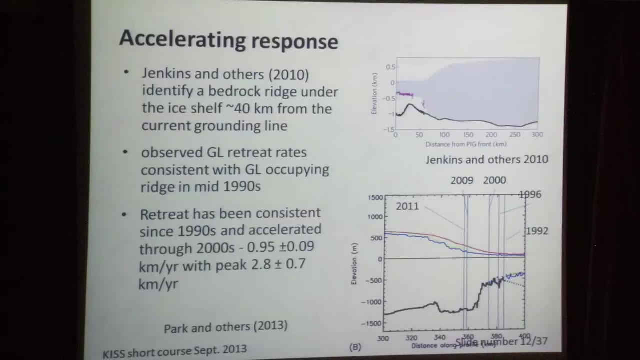 of the ice at this particular location, close to the ground in line, And you can see that there is indeed an acceleration of the rate of mass loss from this glacier. Then the final piece of the jigsaw puzzle was delivered by Adrian Jenkins, reporting the auto sub that we've heard about already, and it 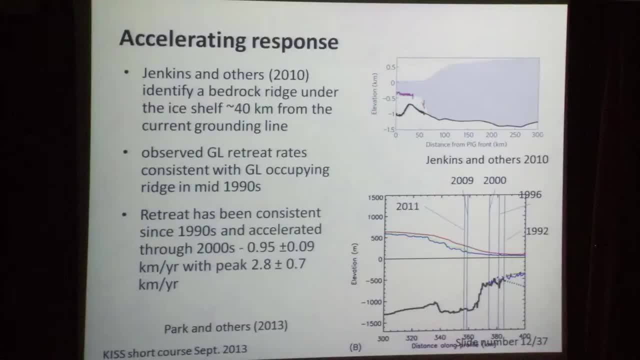 is that it's traversed underneath the ice shelf. Now we've heard that the data collected by Auto Sub on ocean water properties. Auto Sub also carried a bottom reflector so it could map the topography of the bedrock underneath Pine Island ice shelf, which was unknown up until this point, And they discovered a ridge. 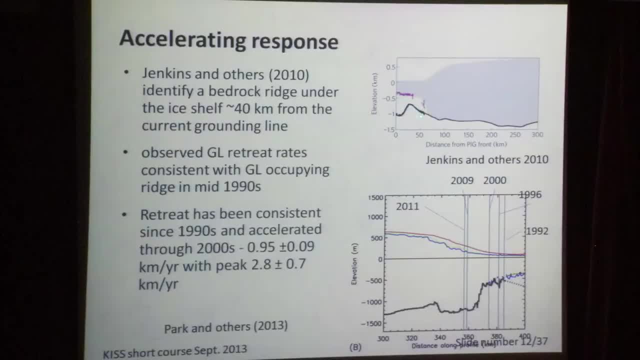 here. So what appears to be happening is that the grounding line now here is from a point of stability- and I'll come on to why that's a point of stability shortly here- And what we're seeing is retreat from that stable point, perhaps down into the main body of this very deep glacial trough And, more recently, a 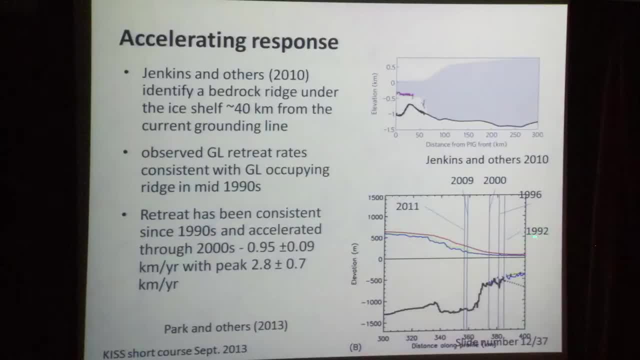 group at Leeds in the UK has mapped the grounding line extending Eric's work going now from 1992 all the way through to 2011.. And you can see the location of this grounding line and its retreat into. this is the bedrock topography here. So this is a peak and we can see that the grounding down is now. 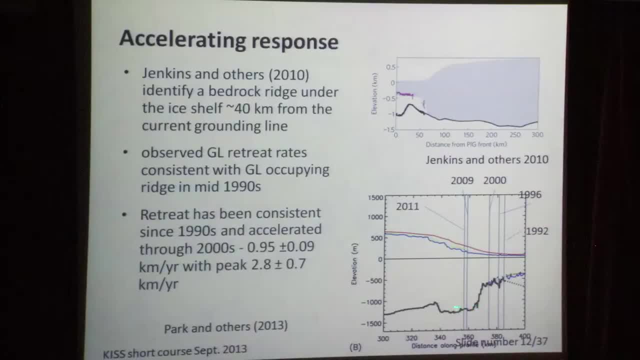 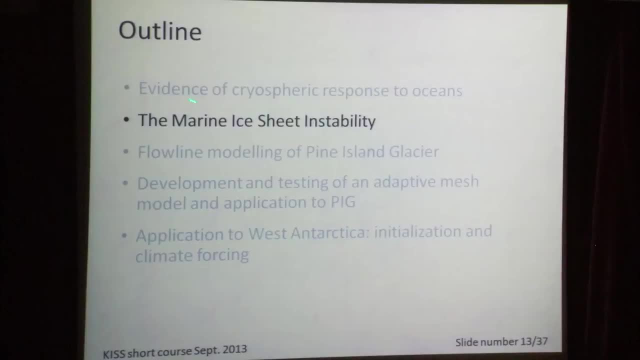 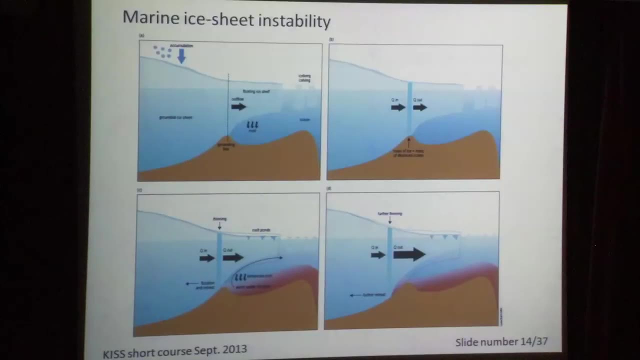 it's quite as retreated right back into this trough here. So why is this important? Why are people worried about it? Because of the marine ice sheet instability. So I'll just say a few words about what that is. Here's a series of schematics. we'll run from a, b, c and d. Here's an ice sheet in. 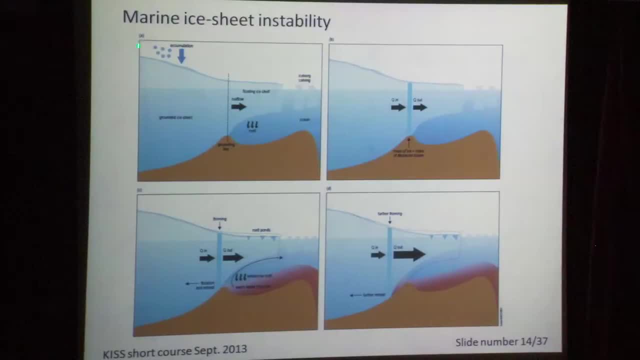 equilibrium where we have accumulation, snowfall flowing, accumulating on the surface of the ice, forming ice flowing out towards the coast and we have the grounding line here. Now for this grounding line to be in equilibrium, the flow of ice reaching the grounding line from the ice sheet. that's going to be the ice sheet. 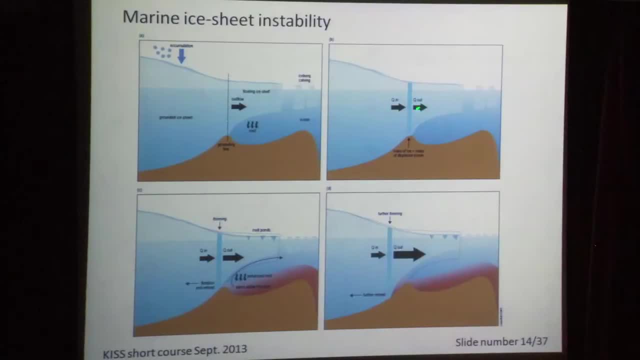 upstream, ie all this accumulation must exactly balance the mass lost into the ice shelf or icebergs or whatever. So this is an example of a marine ice sheet in equilibrium. So what we think may be happening is that, for some reason or another, the outflow from 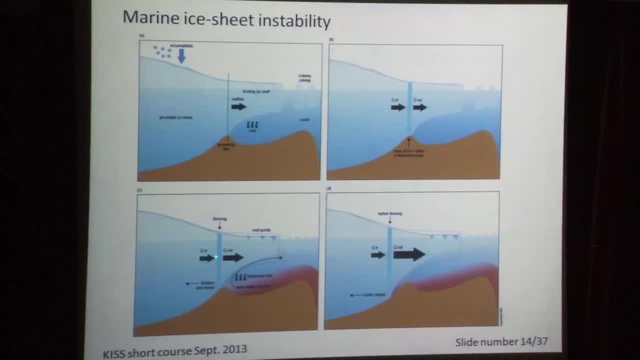 the grounded ice is increasing such that it's more than can be balanced by flow from accumulation. So, with more going out than coming in, this column of ice must thin Because it's floating or it's balanced on bedrock. it will start to float. 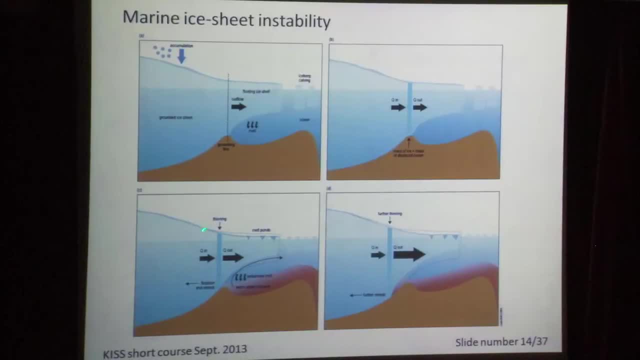 So the grounding line will retreat. Now, why could that happen? Well, we've already talked about two processes. Perhaps the ice shelf is becoming weakened by the existing ice, The resistance of melt ponds, as in the Larsen, or perhaps the ice shelf is becoming thinned. 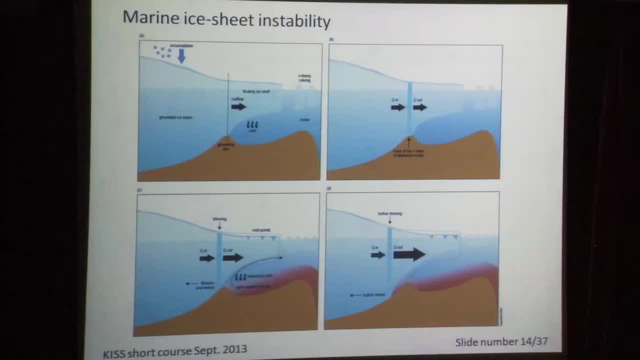 by the presence of warm- relatively warm- ocean waters thin the ice shelf, make it less able to resist the flow of ice. So we now have a case where this column of ice at the grounding line is thinning. It's going to start to float, so you're going to have some retreat. 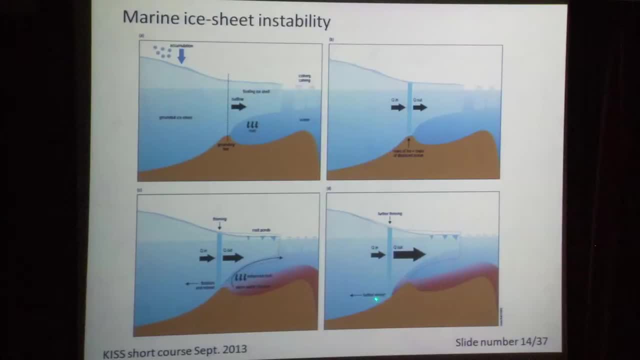 And that's a self-sustaining process now, So that as you're retreating here, the amount of discharge is going to start. it will continue to increase, but you're now in thicker ice, more likely to discharge, So it's going to tend to want to retreat more and the bedrock here is deeper. 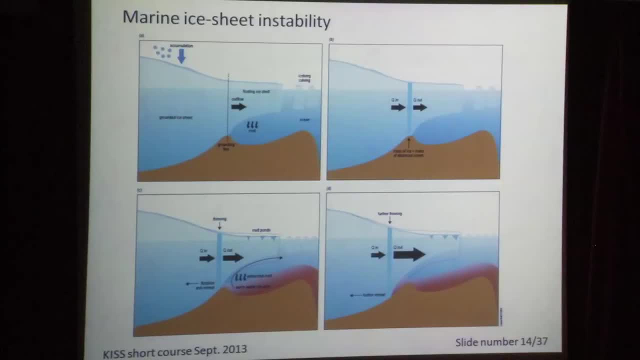 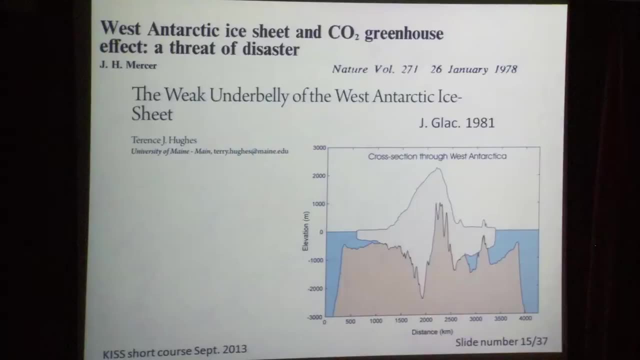 so it's going to be harder for it to float. So that's the sequence of events leading to marine instability, And this line of argument has been around since 78 at least. There's a series of papers And there's a series of papers. 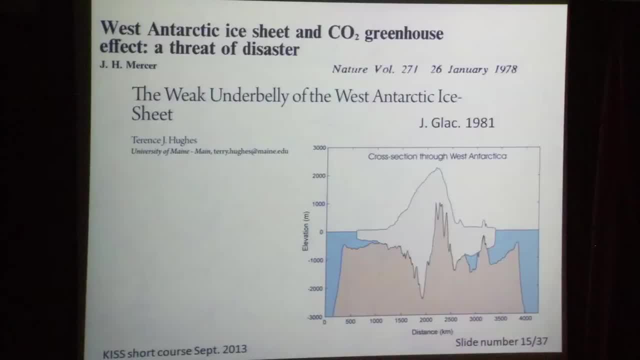 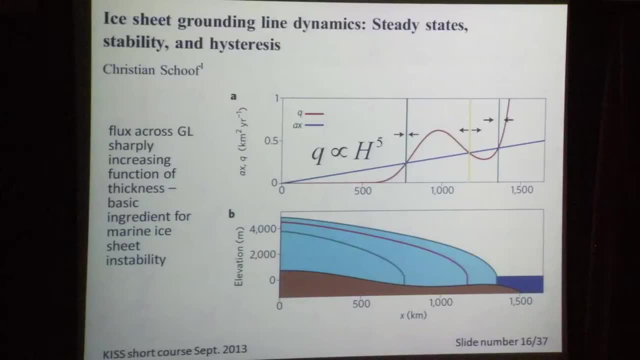 In the early 80s, highlighting the importance of potential importance of this for Antarctica. More recently, Christian Schoof has taken this literature and put it on a more satisfactory theoretical basis. So many of those analyses that I just showed you, or that I alluded to, were fairly ad hoc in their nature. 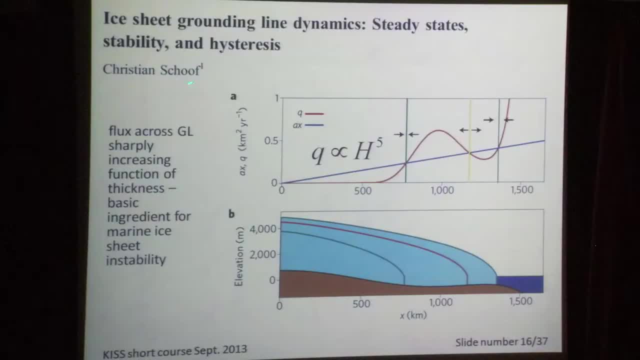 And the step forward that Christian has provided the community. the community is to remove that ad hoc ism and put this theory on a more sound theoretical basis. and here's a key figure from Christian's paper. so we have a very nice shelf ice sheet, rather his bedrock and his ice sheet. there's the 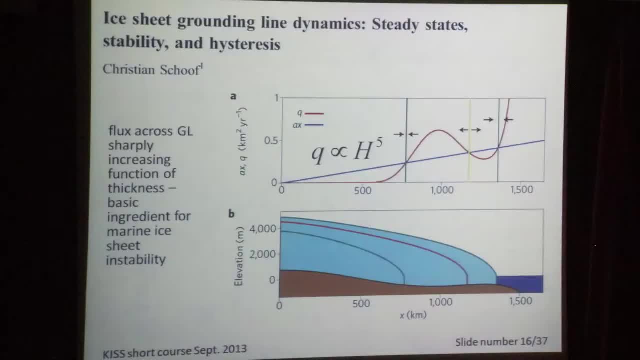 grounding line in this location and in this simple 1d analysis that we're just going to look at steady states, we have in this graph flow at the grounding line in units of flux and here we have distance from the ice divide towards the ocean. and there's two lines here. firstly, the blue line in this simple analysis. 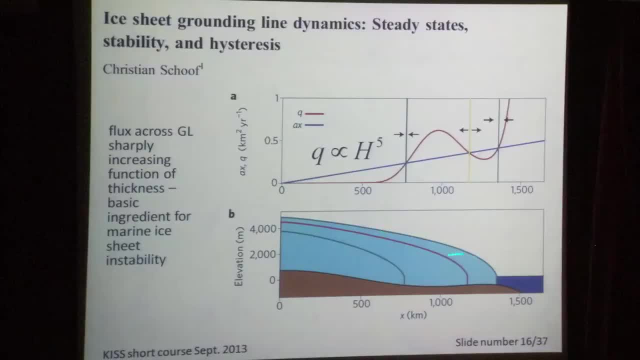 this is going to be the outflow, the masses that has to leave the ice sheet sheet and Christians assuming constants accumulation. so this is just a linear function of distance. as the ice sheet gets bigger, there's more surface area for snow to accumulate. therefore there's more flux to get rid of. in Christians analysis and 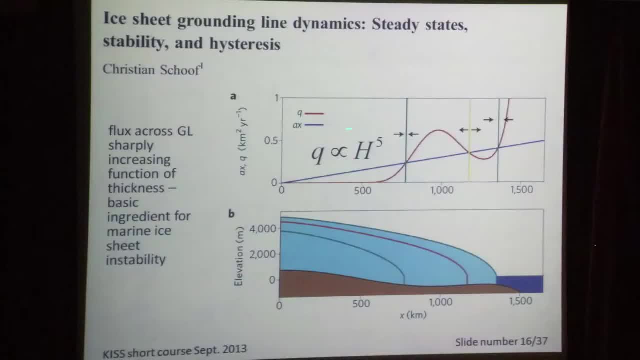 his breakthrough was that he could come up with an analytical expression that related the flux that's discharged across the grounding line as a function of the thickness at the grounding line. now we know the thickness at the grounding line because we know by net definition that the grounding line is. 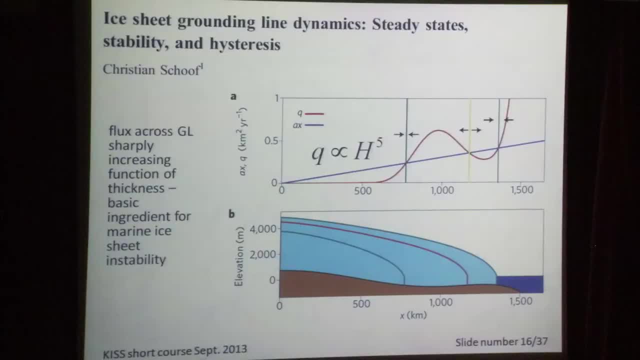 just balancing the ice sheet and the ice sheet is just balancing the ice sheet. that's causing buoyancy. so if we know the bedrock, we know what the thickness ought to be. so you can construct this sort of curve knowing what the bedrock topography is. and there's a number of points of stability here where the two 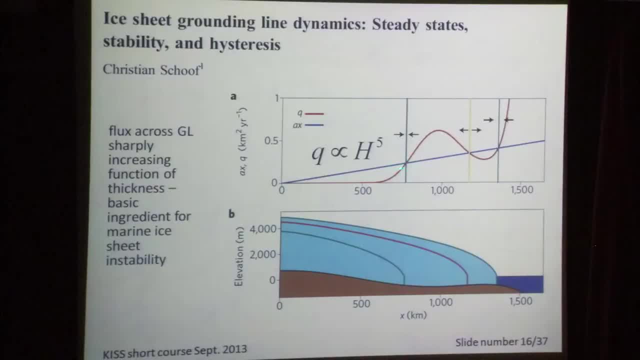 balance. so at this point the two flux is balanced and we're in equilibrium here, here, here, here. if we take this point here and we increase the outflow for some reason, then there's more leaving the ice than being balanced by flow from the interior. So that's a stable point. 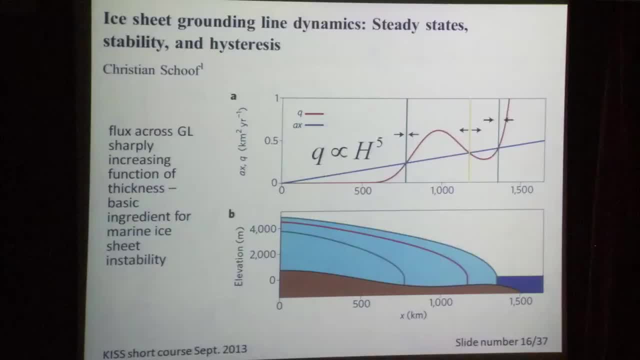 That's going to go back to the equilibrium, So you can perturb it and it will return to the steady state. So it's a stable position. And you can contrast that to this point here where if you increase the flux, leaving the ice sheet. 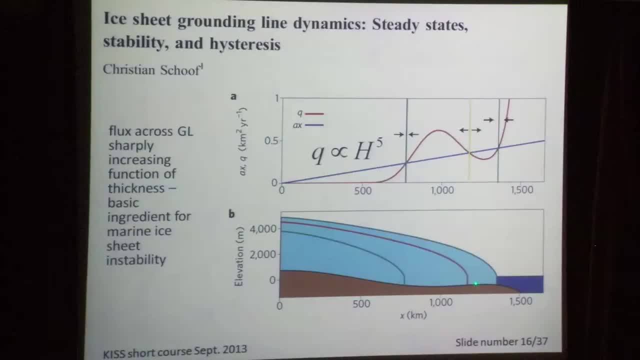 then you can go through this path here and you get an irreversible retreat back to the next steady state. Now, this is a theoretical analysis, And while it's fantastic in that it sets the ground for us, it can't be used in predictive modelling of Antarctica for two reasons. 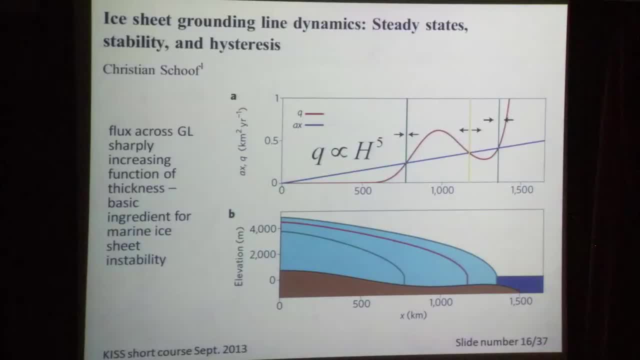 Firstly, it just deals with steady states. It doesn't tell us how quickly those steady states will emerge. And secondly, it just deals with a one-dimensional ice sheet, So it doesn't include things like butchering from ice shelves. That's why you need numerical modelling. 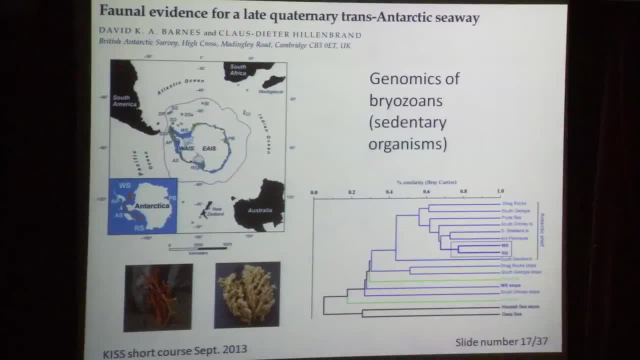 I thought I'd just throw this one in because I was just struck by the interdisciplinarity of this. So we come up with the idea that West Antarctica may be potentially unstable, And I was just struck how interesting this work was. 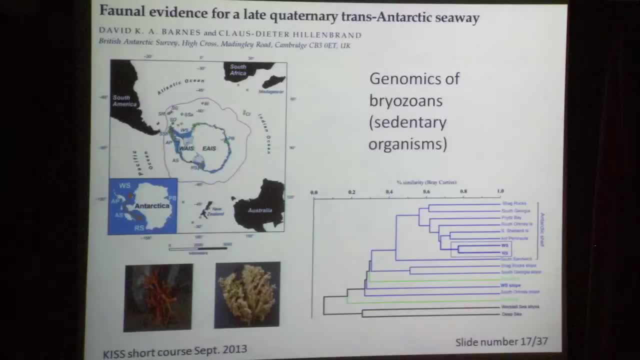 So the question then is: how can we gather data to test that idea? This particular A group of workers have used the genomics of bryozoans, which are sedentary organisms at the base of the on the sea floor. 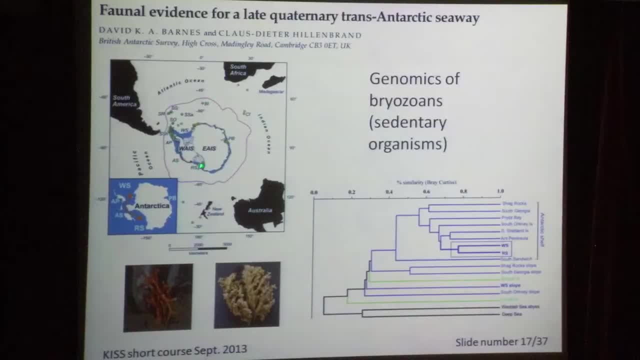 and looked at the genomics of various communities around Antarctica and found that actually the Ross Sea and Weddell Sea communities are very closely aligned in their genomics, suggesting that they must have been talking to one another very recently, perhaps during the last interglacial 120,000 years ago. 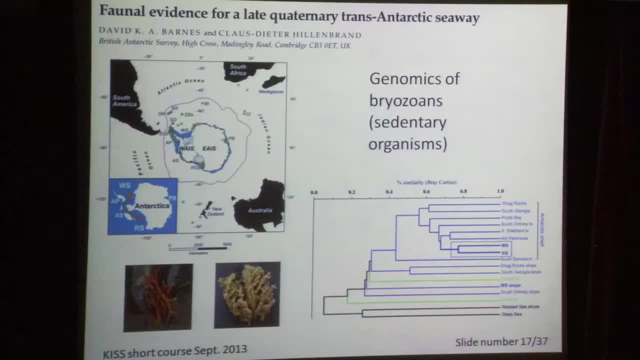 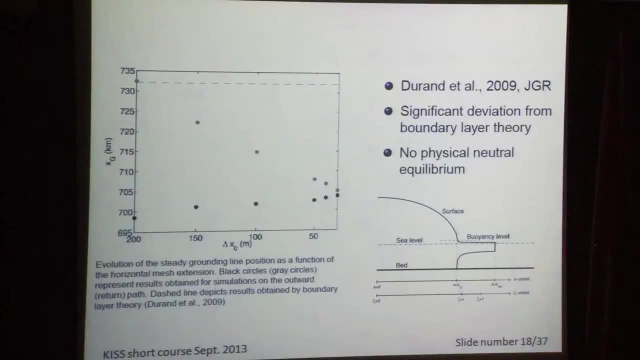 I'll just put that in As an aside, because I was struck by how interesting it is to use different tools rather than the usual geophysical tools that we employ. So, coming to numerical modelling of ice shelves and ice sheets and grounding lines, indeed, 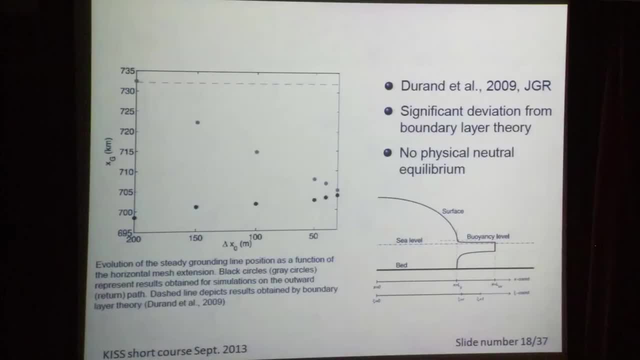 On the face of it, this is what you ought to do. However, there's a body of work over the last five years or so that's suggested that if you do this, you have to do it with great deal of caution, And that's because the results turn out to be highly dependent on the grid spacing that you employ in the model. 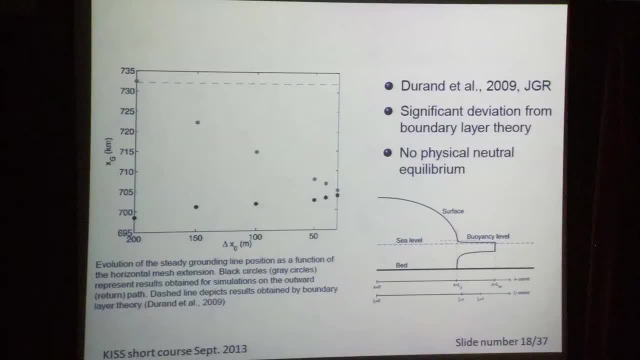 All numerical models have some sort of representation of space, of grid spacing, And in this paper by Gail Duron he showed that the grounding line position depends quite sensitively on the grid spacing. So he only gets convergence around about 50 metres grid spacing. 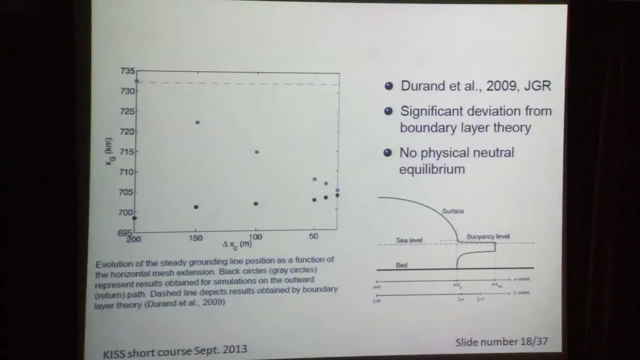 Now we're proposing to use this sort of model for all of Antarctica. So clearly, 50 metres resolution is an impractical proposition. Indeed, 200 metres is an impractical proposition. Most models would typically use something like five kilometre grid resolution. 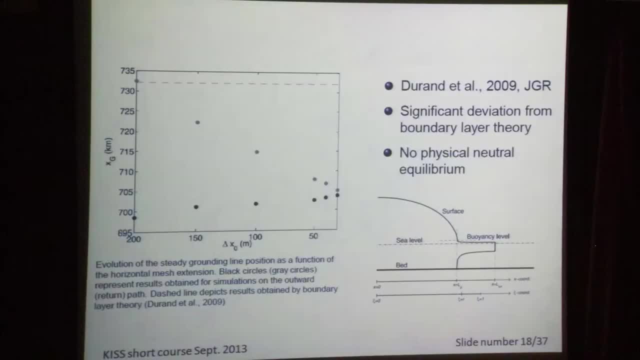 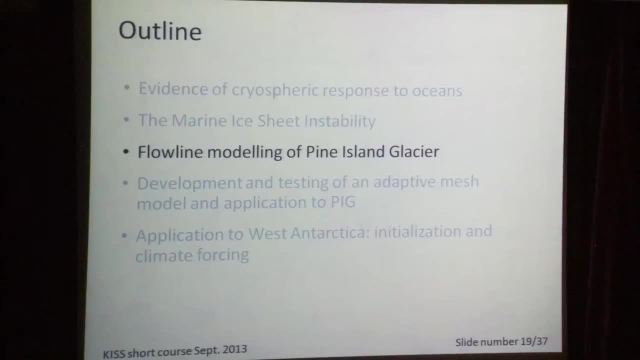 So this is a severe challenge to the type of numerical models used to predict what's going to happen. So now I'm going to turn to work that we've done on Pine Island Gathsea and predicting its future, And indeed it's passed. 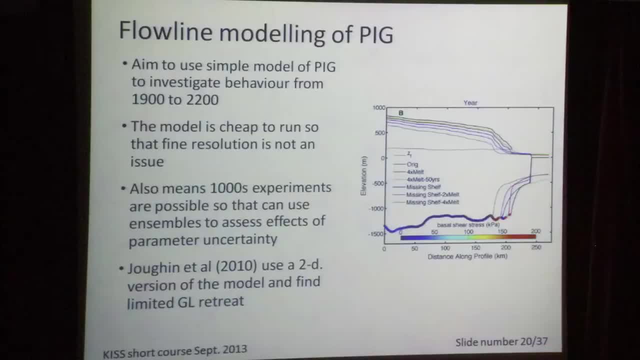 We were beaten to this by Ian Jochin, who in 2010 published some finite element modelling of the future of Pine Island, Glacier, And he found that actually wholesale retreats in the marine instability type mode doesn't occur And he reaches a point of stability, the grounding line retreats, but only 30 or 40 kilometres. 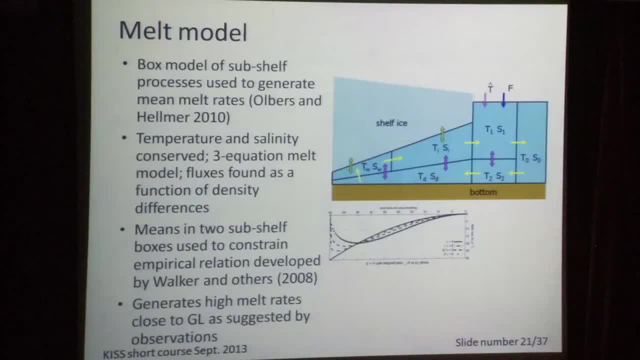 So our work was set up to test that, And what we developed was a toy model, a flowline model of the Pine Island system that included a box model of melt rate calculations, So it had the three equation model in it And it had conservation of temperature salinity in the cavity, but in a fairly cartoon fashion. 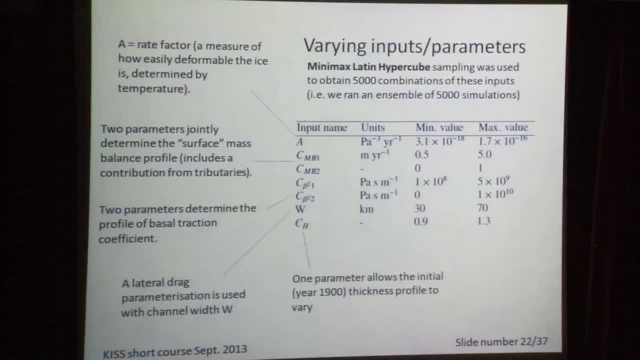 And the idea is to force that model with a projection of ocean temperature To see what happens. The advantage of having a small flowline model that's easy to use is that you can run it many, many times. So we ran 5,000 different combinations of these parameters, which relate to ice flow and geometry. 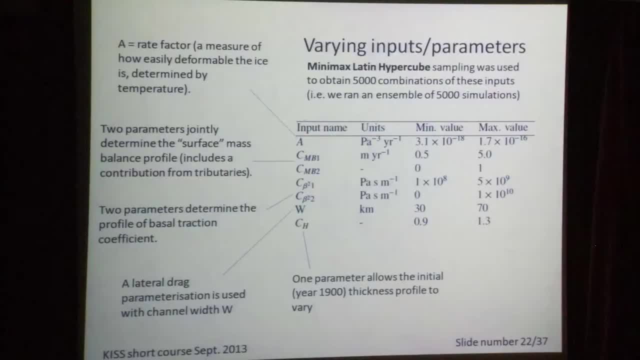 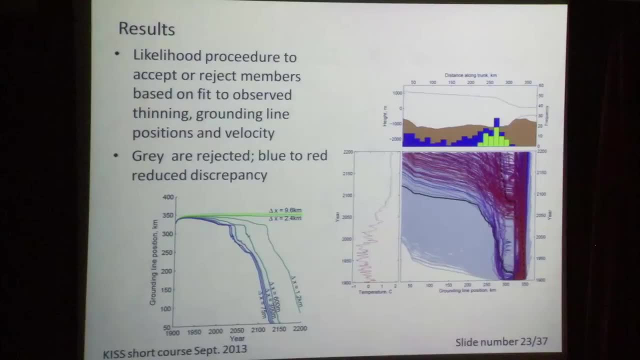 All the unknowns that we have on the ice sheet side of the equation And the results are shown here. So it's quite a complicated figure. Here's ground in line position, So currently it's there And then it may retreat in the future. 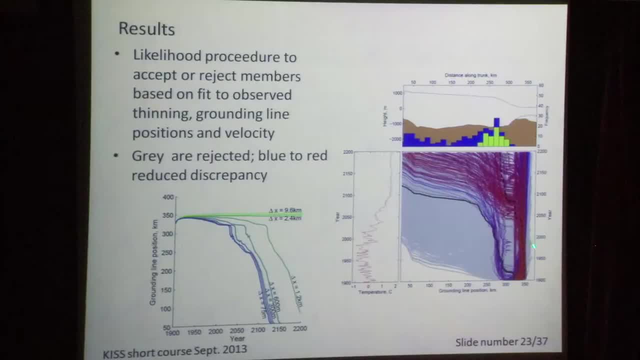 This is time going from roughly the present day there up for two centuries, And these individual tracks just show you, for a particular model experiment, the ground in line location. Now you'll see that some are in grey and some are in red and blue. What we could do was use a comparison to observational data. 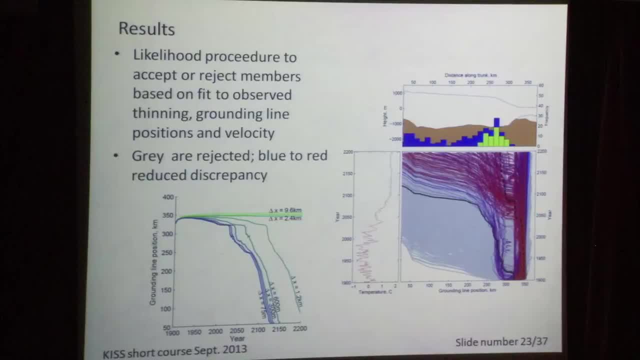 To test which of these 5,000 experiments satisfied the criteria that they agree reasonably well with observations. So that's why the bulk of these grey ones are ignored, Because they don't pass that particular test. But what we do get is two sets of types of experiment. 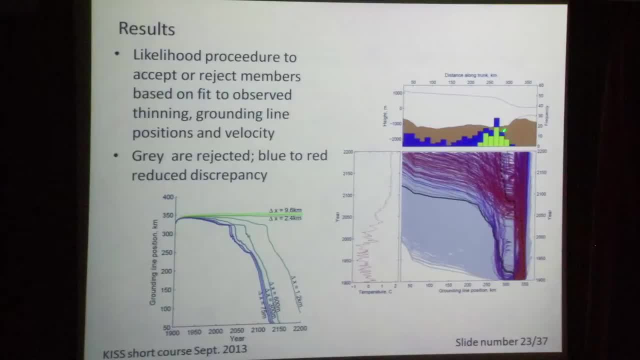 One in which we get a ground in line, stabilising in roughly the position that Ian found, But also we got a larger ground in line, stabilising in roughly the position that Ian found. But also we got a larger ground in line, stabilising in roughly the position that Ian found. 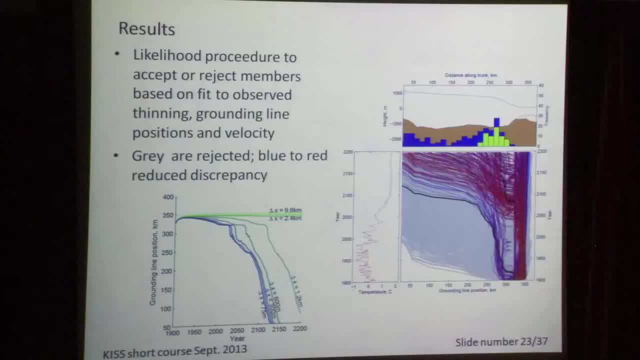 And a large group that continues to retreat up the whole of the trough Such that there was no ice left after by 2200.. So David was talking about parameter uncertainty. essentially, I think it's clear that a lot of these parameters matter to ground in line retreat. 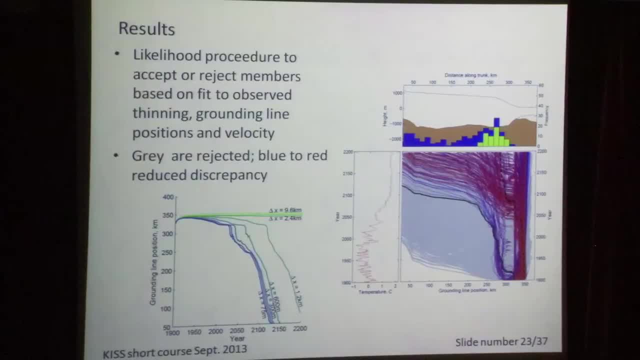 A lot of the parameters associated with ice flow and indeed what we know about the ocean circulation underneath the ice shelf, A lot of the parameters associated with ice flow and indeed, what we know about the ocean circulation underneath the ice shelf, And it seems that, whatever we do, 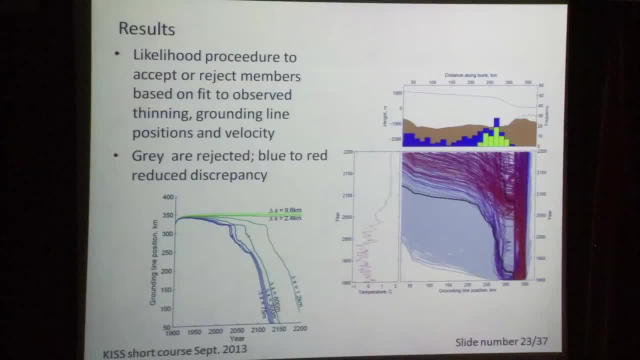 we need to do modeling in this sort of framework, So we're assessing the uncertainty of those parameters that are making some sort of probabilistic prediction, rather than just trusting one particular model. We note that our flow line model is. the results are heavily grid dependent. 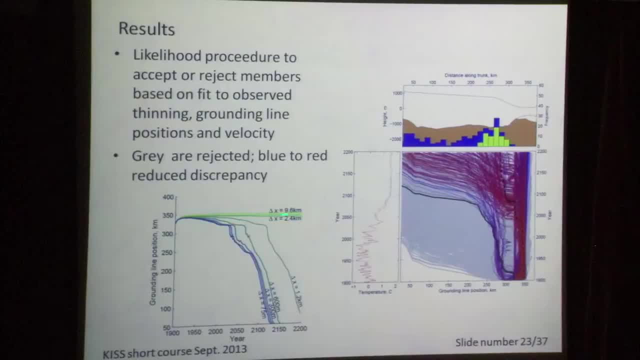 So we can run the model at 10 kilometers, two and a half kilometer resolution, and nothing happens. It's not until we go down to sub-kilometer resolution that we get some sort of convergence. So around about 75 meters. 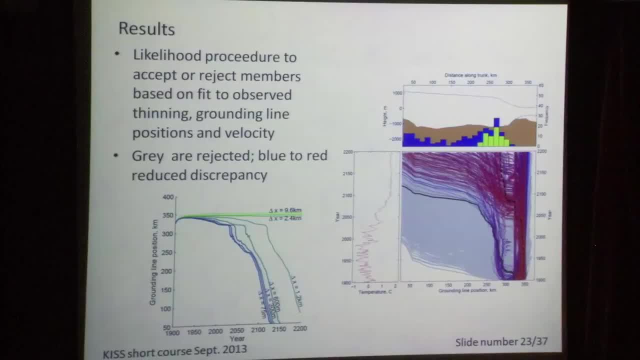 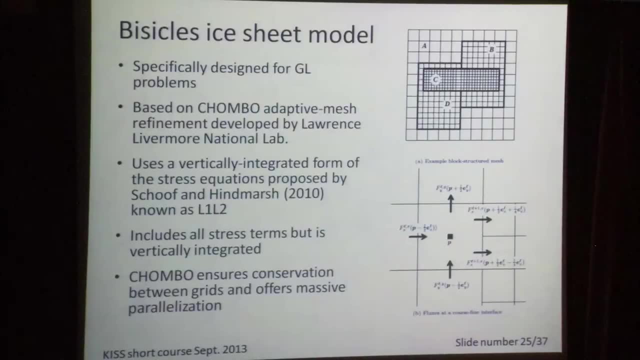 300 meters grid resolution is required to capture this process. Now, taking that understanding and applying it to a full-scale model of Antarctica is a challenge, because we're now fairly convinced that we need high resolution near the grounding line, least sub-kilometer. perhaps better than that. 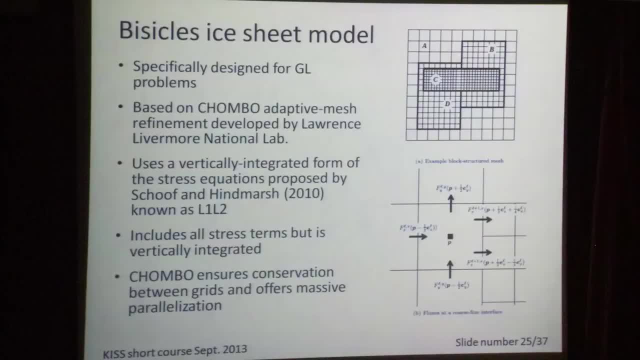 So what our effort has been in the last five years or so is to find a method of delivering that. It's clearly impractical to model the whole of Antarctica at that sort of resolution, So we require some sort of adaptive mesh software. 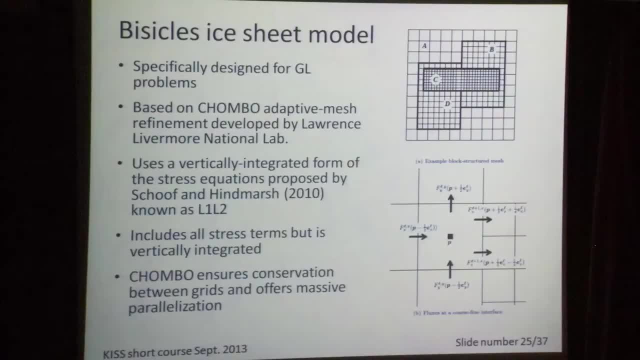 We made the decision that it's easier to write an ice sheet model than it is to write an adaptive mesh model, So we scrapped the ice sheet model and took on board this framework that's been developed over the last 20 years by the. 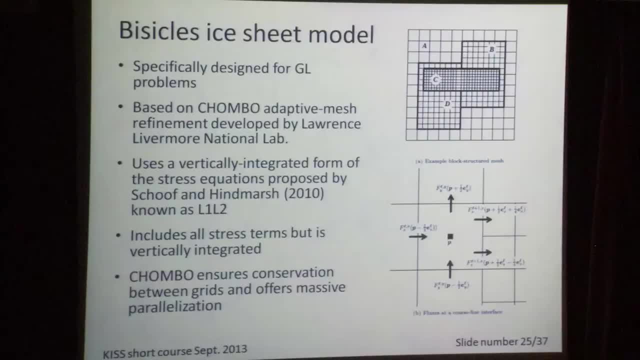 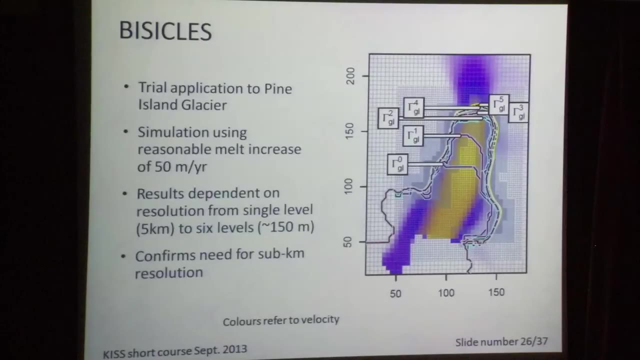 Livermore National Laboratory. Lawrence Livermore National Laboratory originally developed for nuclear explosions and the like, but does all the adaptive mesh business for us. So we've built an ice sheet model within that framework. In the trial applications- again, it was indeed the case that. 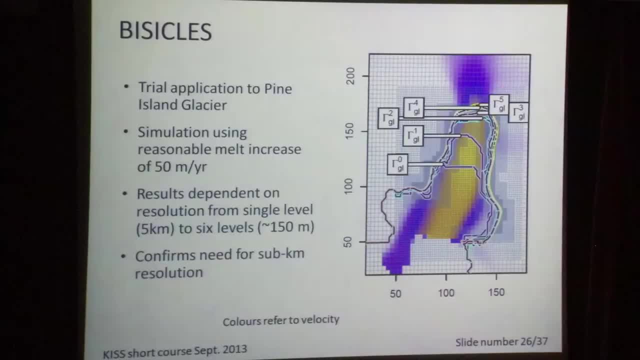 the predicted migration of the grounding line, heavily dependent on the grid spacing that you use. So here's an illustration of how the adaptive meshing works. We have a criteria that essentially says if you're near the grounding line, you need to find mesh. 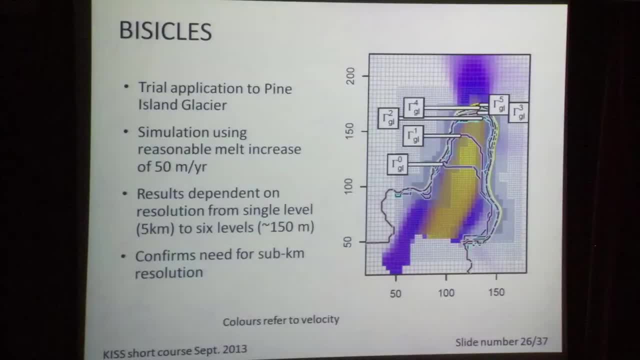 and you can see that these meshes sit within one another. Trombo takes care of all of that. What we're showing is the grounding line position for various mesh sizes. So the base mesh is five kilometers and if we apply a substantial perturbation to melt rates, 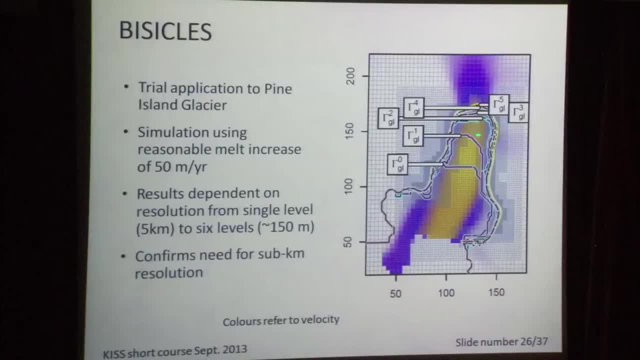 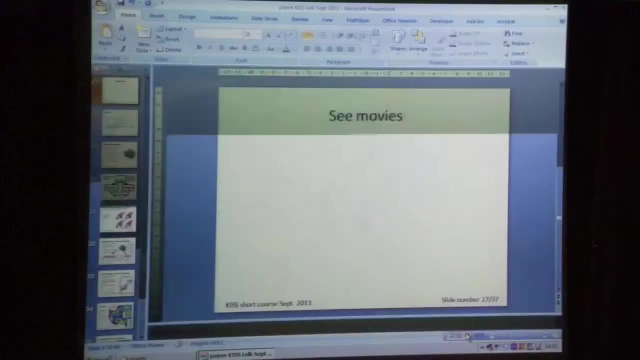 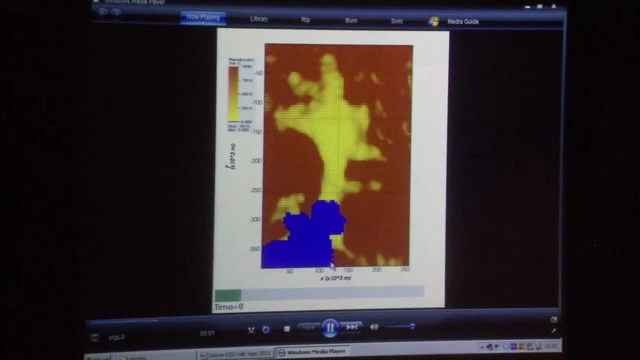 the grounding line is anchored at this point it doesn't move. So only when we start using different meshes that we get the grounding line to move. Now, I'm not as sophisticated with movies as David was, so I can't embed them, but I can show them to you. 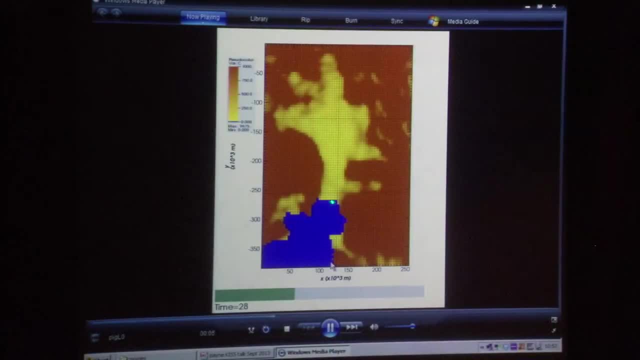 So this is that model experiment. This is the uniform mesh. at five kilometers We're applying an increase in melt rates to the ice shelf and nothing much is happening. So if we didn't know about this issue, about grid resolution, we'd say: Pine Island is stable. 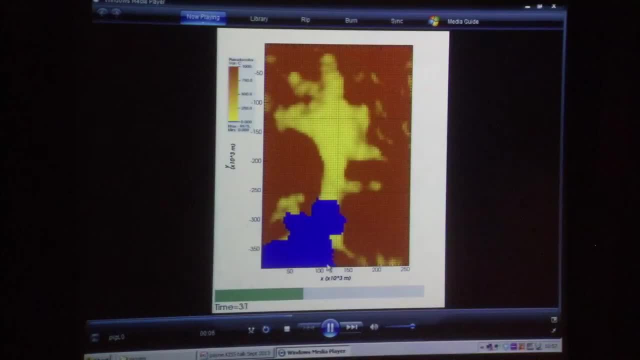 we don't have to worry. This is an example with four levels of mesh refinement, exactly the same forcing as I've just shown you. So we're down in the finest mesh to below a kilometer, probably about 500 meters. So you can see the response to exactly the same forcing is very 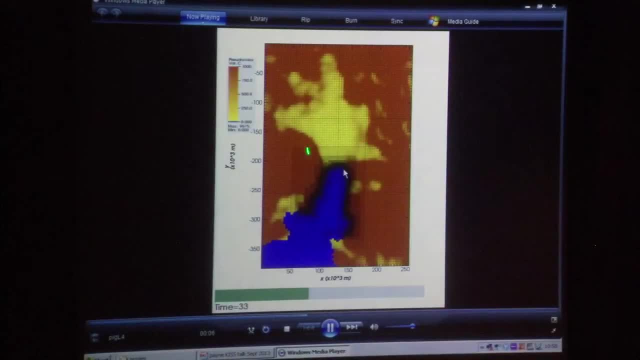 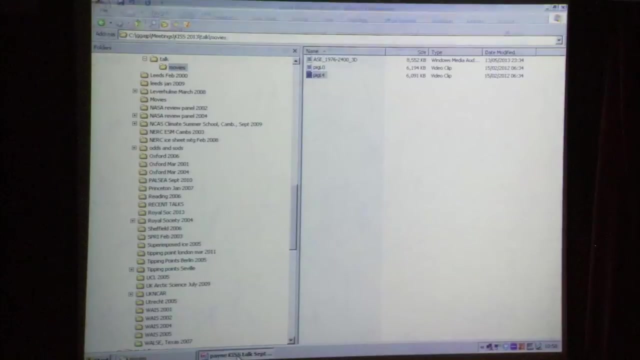 very different and it's actually more akin to what that flow line predicted of large-scale deglaciation. That's years down there. So well, there is a choice and the algorithm just looks to see whether the ice is floating or how close it is to floating. 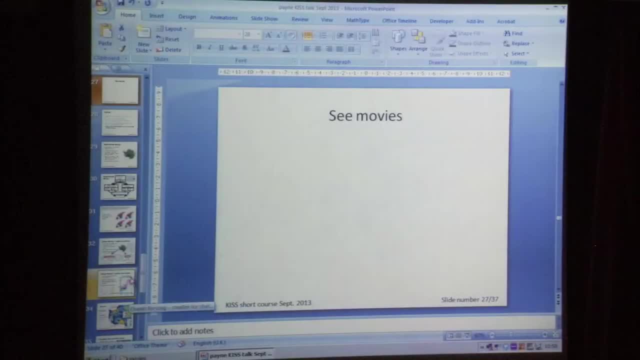 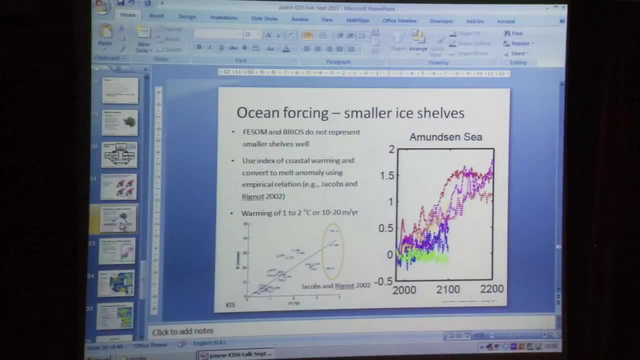 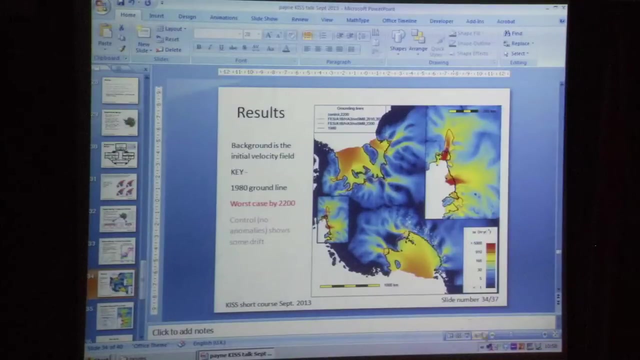 Okay, I've just got. I probably won't manage all of this, so I'm going to skip to the end, to the punch line. So one can apply this sort of technology to all of Antarctica. This was done within the framework of 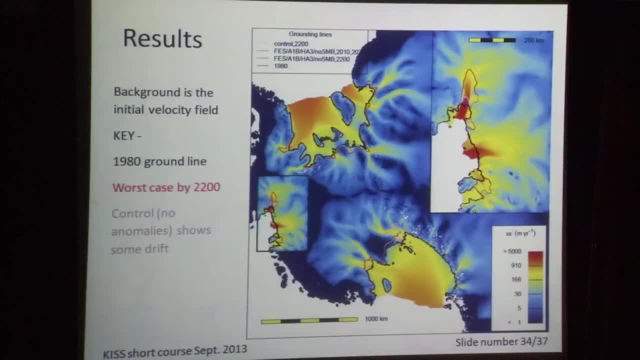 the European Union ice to sea project, where we collaborated with a group from Utrecht to provide projections of snowfalling and we adapted the Washington33,, which was a dead ice to certain degree, to a quarter of what the current normal climate. 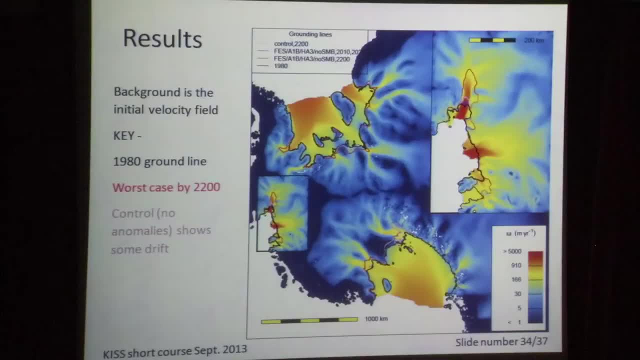 would look like because the edges would change. Of course you've got the Arctic Ocean. that's very low and we cut that down because we thought that that would increase, but, more importantly, with the Alfred Wegener Institute, who used their regional model of the southern ocean. 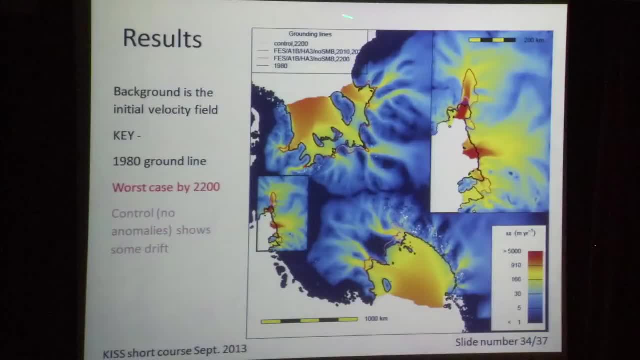 to look at what may happen to melt rates and ocean temperature warming in the future, And you'll probably be aware of a paper by Hartmut Helmer- I think it was in Nature a couple years ago- and his key result was that data set plus other data for Pine Island on the warming. I think that model 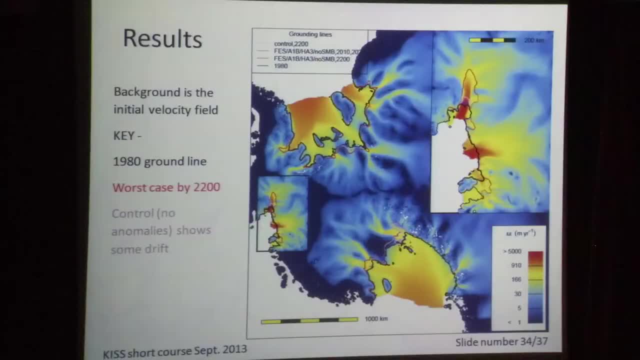 predicted ocean temperatures in the area around Pine Island to increase by two or three degrees or something like that, which is essentially circumpolar deepwater. sitting in Pine Island all the time Now you can just about make out the grounding line, current one in black, and then what I've shown or what we have. 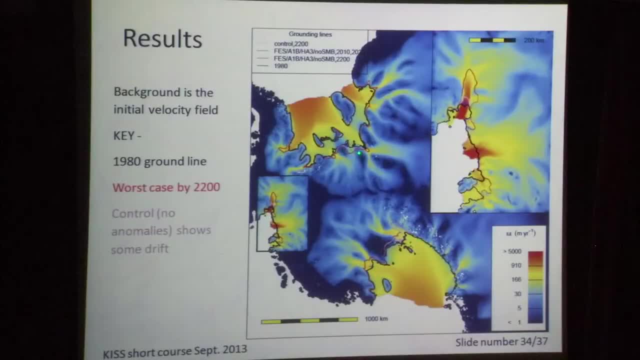 shown are grounding lines at 2100 end of the century and there's a red one and there's a pink one. Those are just different combinations of ocean forcing. So you can see that there is grounding line retreat, very extensive retreat around this ice shelf, the Ronny Filchner, a little bit of retreat in the 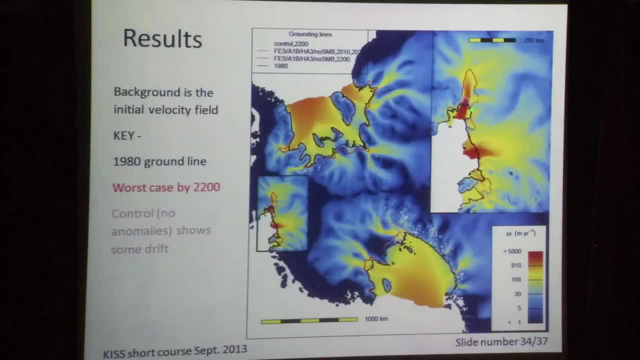 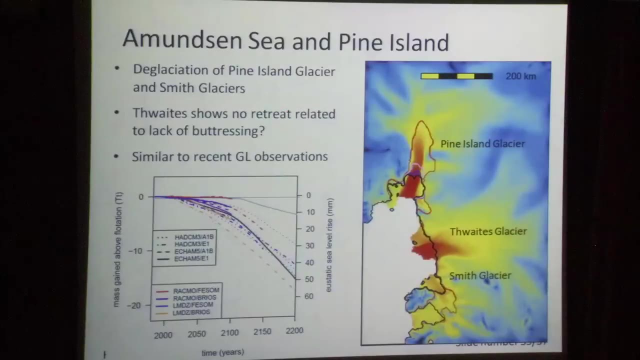 Ross and, in this particular experiment, Pine Island goes, but Thwaites remains pretty much stable and Smith also retreats. Now, because the only thing that happens is Pine Island is lost and this becomes an ice shelf. the actual contribution to sea level is not great, measured in tens of minutes, centimeters or so, and 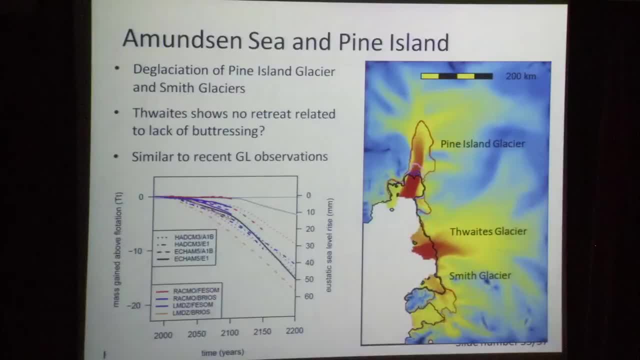 these experiments predict that Thwaites won't do much, and I'll explain why. that is probably in questions, but it's important to stress that's a matter of time scale here. this is just for the first hundred years or so. I'll show you another movie to whet your appetites on the longer-term evolution of the system. 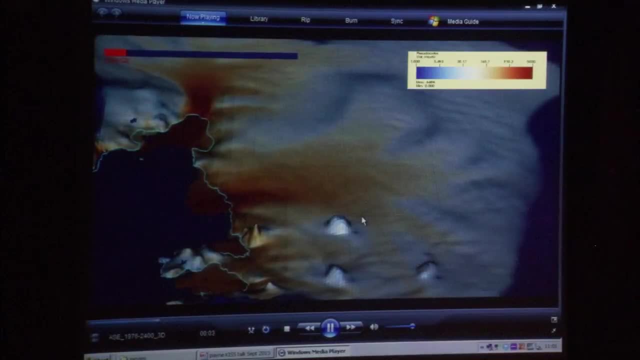 which is here. So this is Pine Island, this is Thwaites, this is Smith, this is Thwaites' Ski heute, and we are playing an ocean warming based on the pheasant work from Arvi. So we can see that Pine Island's grounding line does indeed retreat.